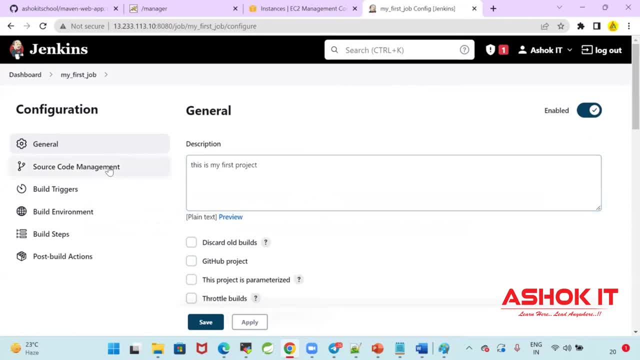 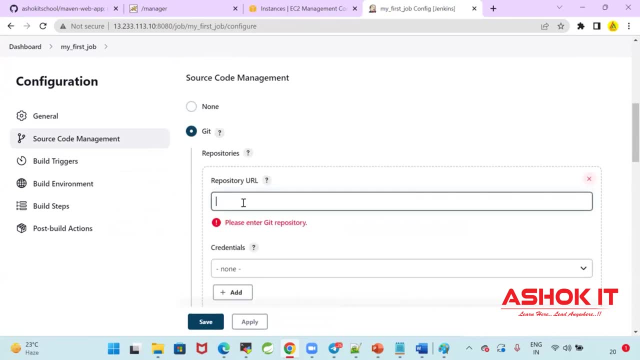 is my first project source code management. source code management. where is the project project is available in the github. na select the git option. give the repository URL. this is my project repository URL. copy this. copy this repository URL and give here repository URL. if it is a public repository, no need. 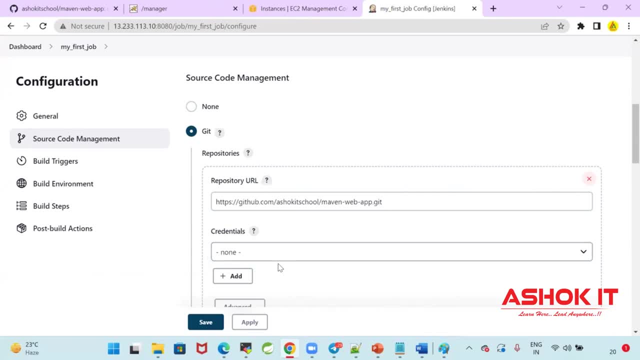 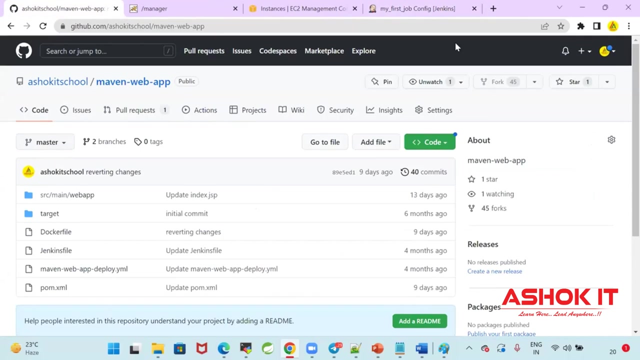 to give the credentials. if it is a private repository, we need to give the credential. my repository is a public repository anybody can access. ok, now I'm giving the repository URL. no need to give the credential in the repository. can you see the branch name? my branch name is a. 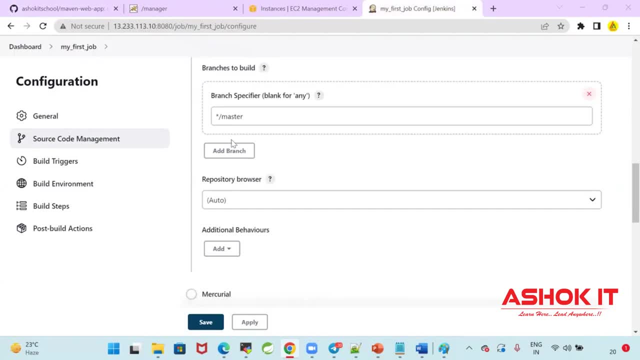 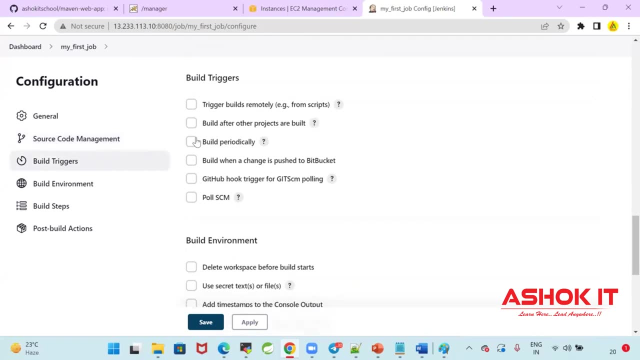 master. if your branch name is different, you need to configure the branch name correctly. my branch name is a master, no problem. then build trigger trigger: build remotely or trigger build periodically. trigger the build when you want to execute the build. that is, you can configure as a build trigger. I am NOT. 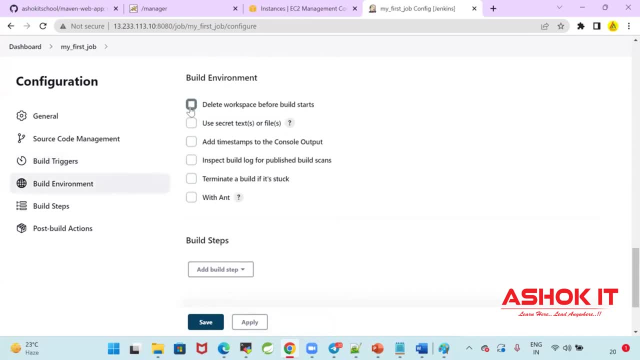 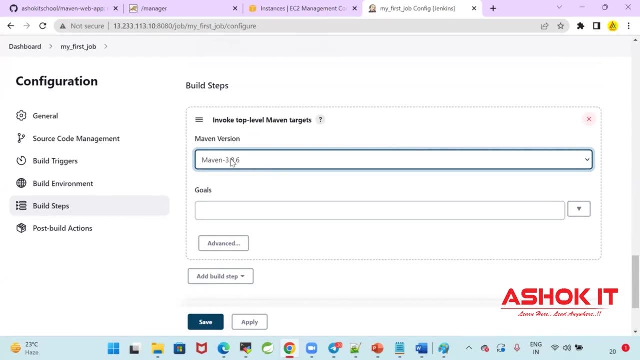 selecting anything: build environment: delete the workspace before build. start previous builds. I want to delete build step. how you want to do the build: execute maven. goal: build step. maven version. select the maven which we have configured in the global tool. in the global tool I configured as a maven, then goals. I want to execute clean. 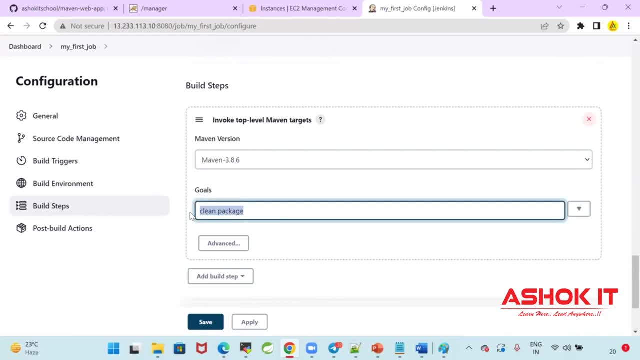 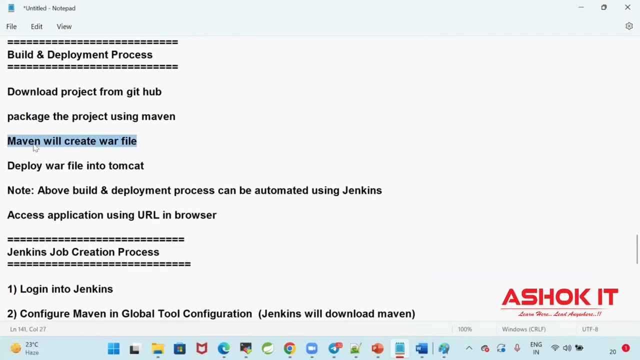 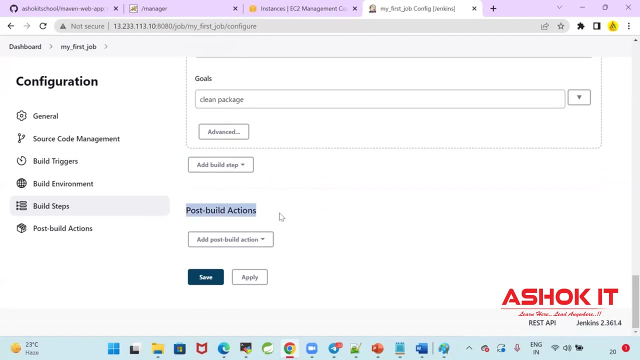 package. I want to execute the goal as a clean package. ok, so with this, maven project will be packaged. maven project will be packaged. it will create a war file. after creating the war file, I want to deploy, that is, post build action. so, general section, a description, source code management from where it has to take the code. I'm 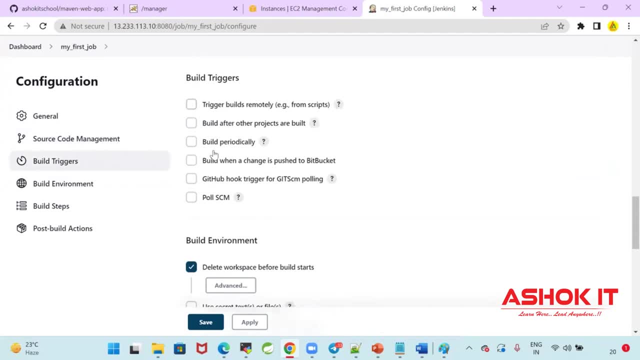 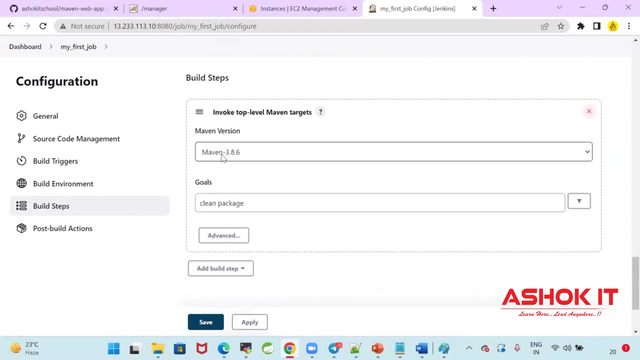 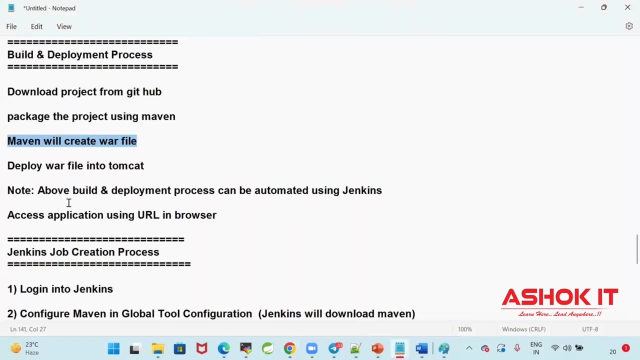 giving the repository URL build trigger when this job should execute. I'm not giving anything. build environment: delete the old builds. build step. execute the maven goal. clean package goals. it has to execute. post build action after war file is created. what you want to do? I want to deploy the work to tomcat. deploy the war. 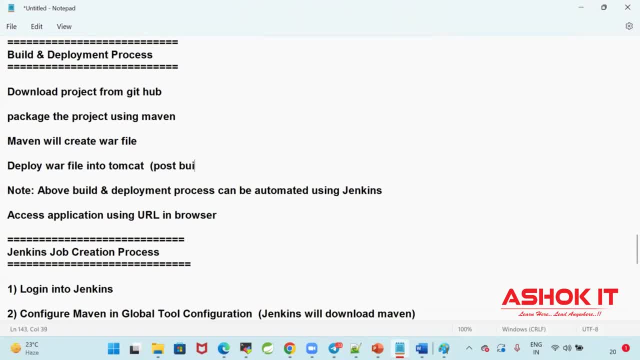 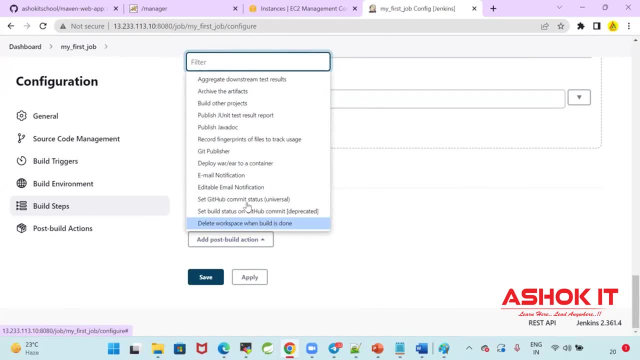 file to tomcat. this is called post build action. this is my post build action. click on post build action. what you want to do as a post build: deploy the bore file to a container in the post to build action and selecting the option called deploy war file to a container. so what? 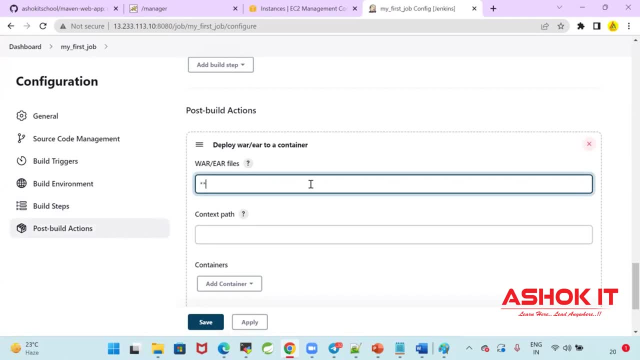 is the war file. what is the name of the war file? my war Negar available inside the target folder, target v Fei available. deploy the warfile to the server. what is the context path? i'm giving context path as maven web app. name of the project: warfile, where the warfile warfile will be available inside the 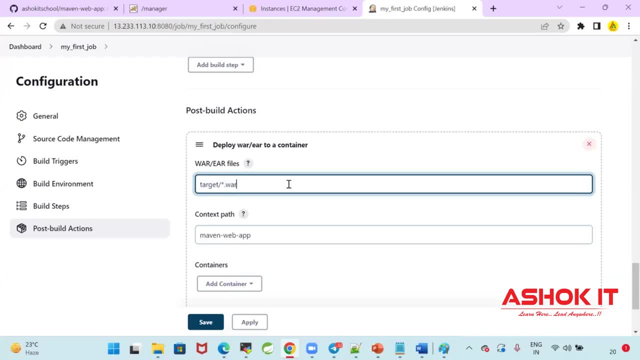 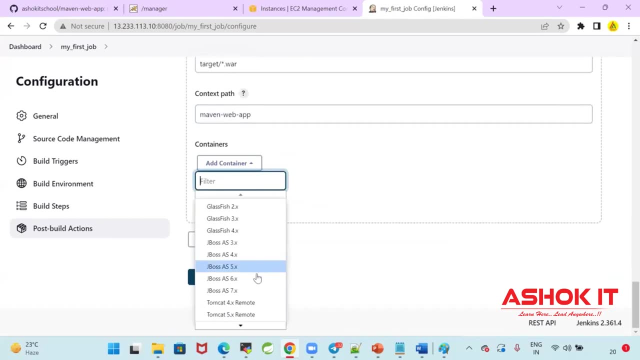 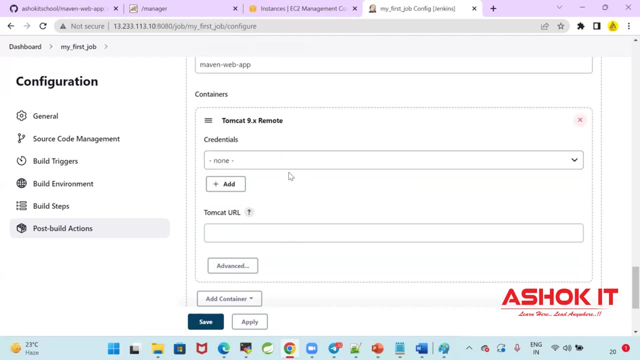 target folder warfile will be available inside the target folder. okay, context path map container. deploy the project to container. which container? i am having tomcat 9.x, so selected tomcat 9.x credentials of the tomcat. so to deploy the project to the tomcat tomcat credentials: tomcat. 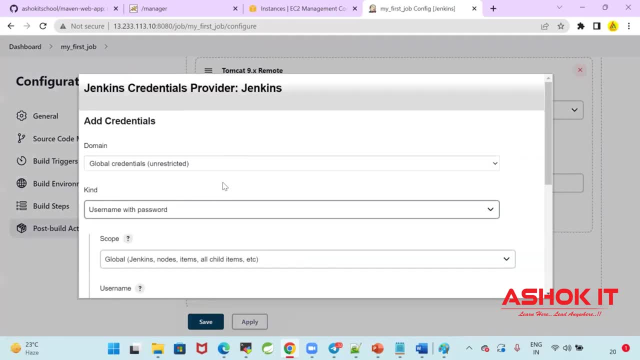 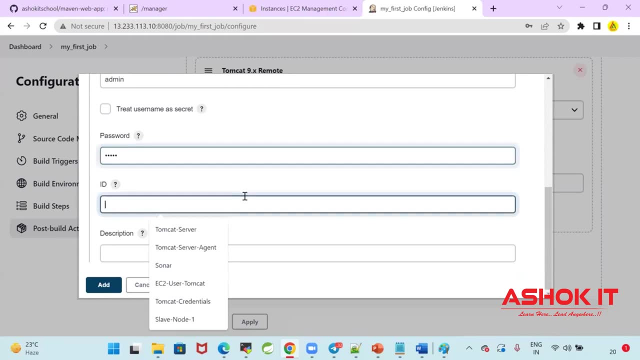 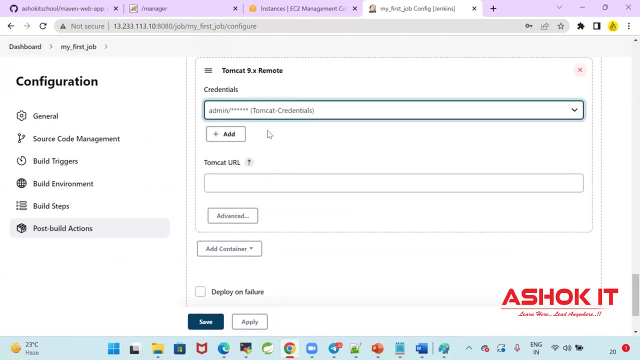 url. i have to configure. add the tomcat credentials. my tomcat credentials are admin, admin, admin, admin is the credentials of my tomcat. i'm going to configure tomcat credentials. add them, select it. these are the tomcat credentials: tomcat url. where is the tomcat server running? tomcat server running. 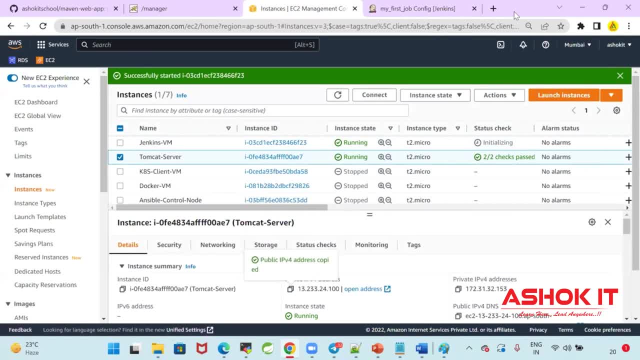 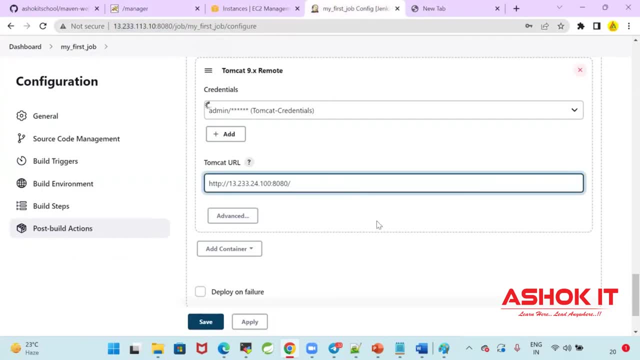 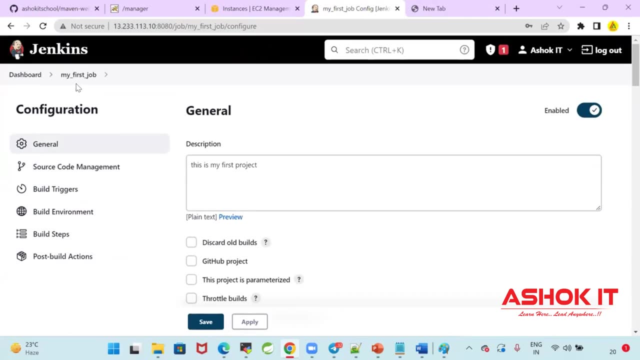 in the cloud. take the url of the tomcat and configure that url. this is my tomcat url. take this url, give the tomcat url in the jenkins. that's it. that's it. see the options i have given. i am creating a first job in the jenkins to automate the build and deployment. this is my first project source code. 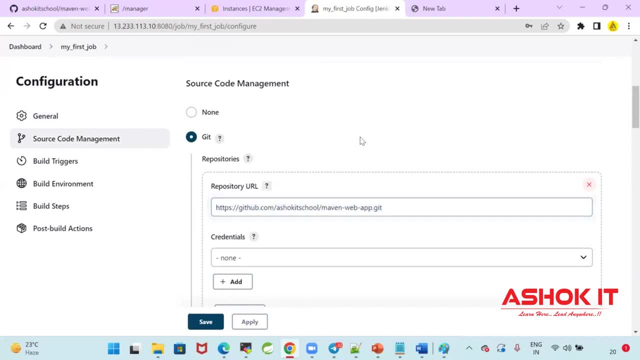 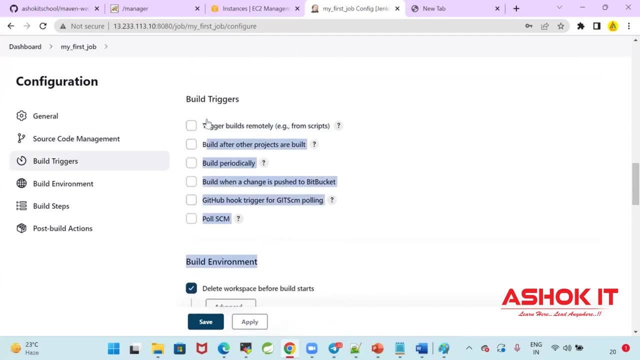 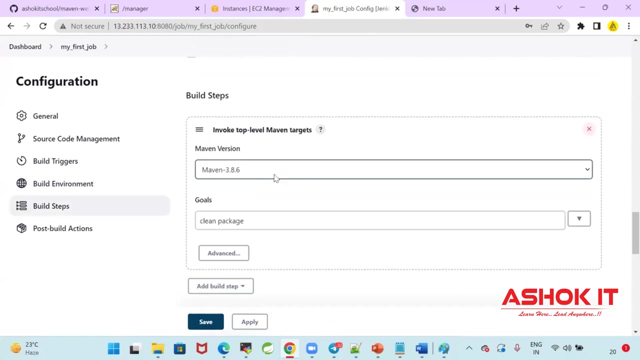 management. i'm giving as a git repository url. it is a public git repository. no need to give the credentials. build triggers: i'm not giving any anything for build trigger. i will tell you what is the build trigger, how to give it. then build environment: delete the workspace before build starts. build step: i'm asking the maven to build. 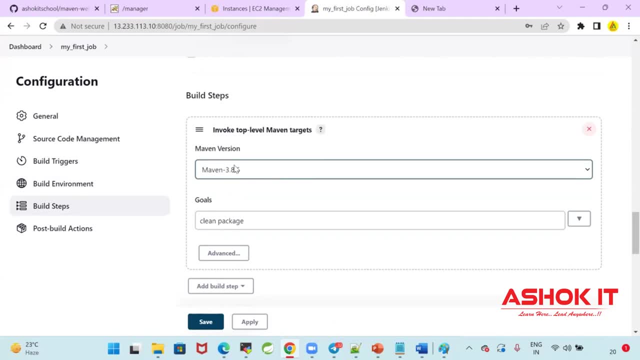 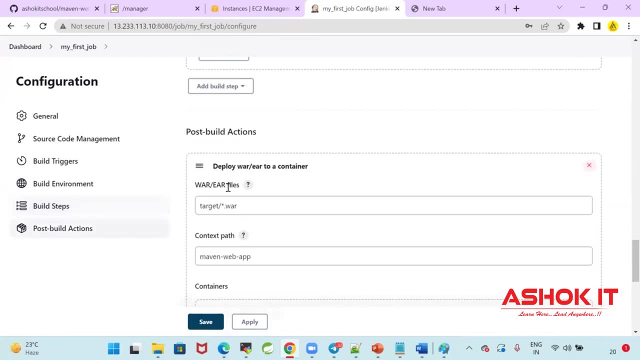 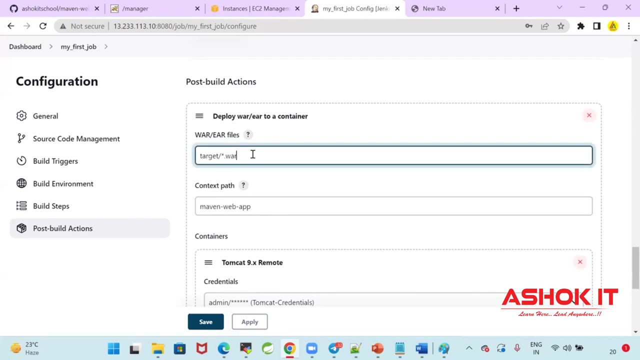 maven i installed as a global tool. i'm selecting the maven, then i'm giving the goals to execute: clean package. package goal will create the project as a war file post build action. i'm telling the map jenkins to deploy the war file to tomcat. deploy the war file to a container. this is the. 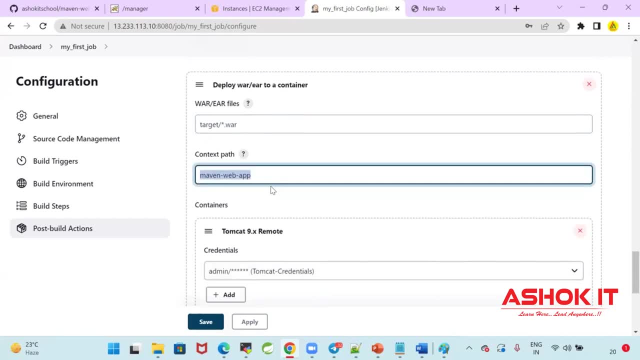 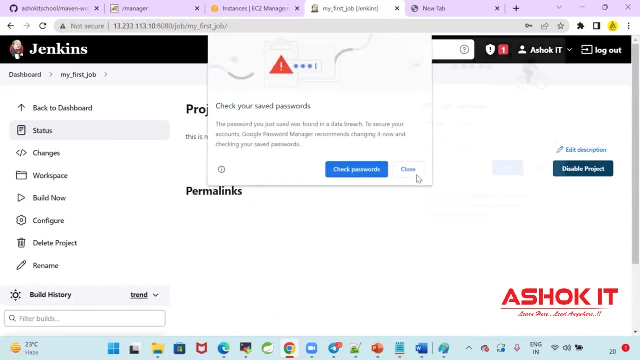 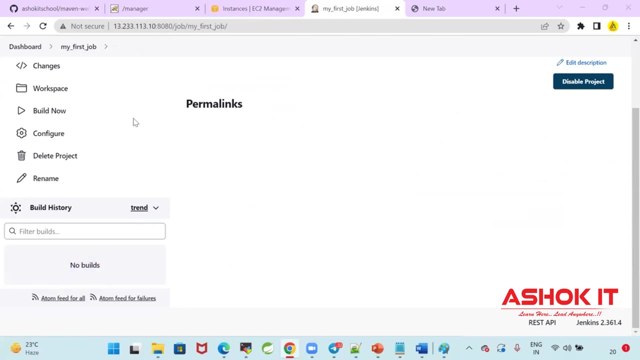 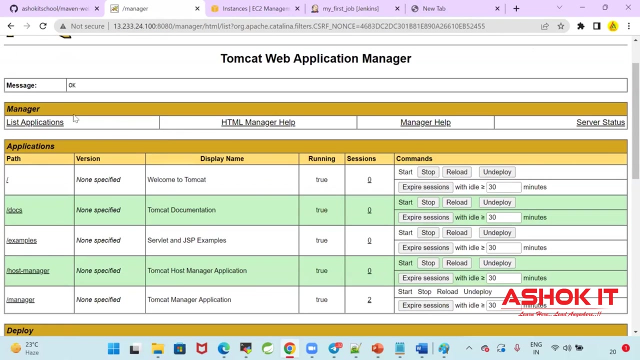 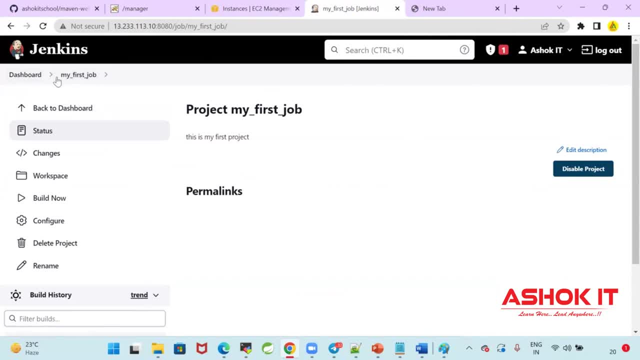 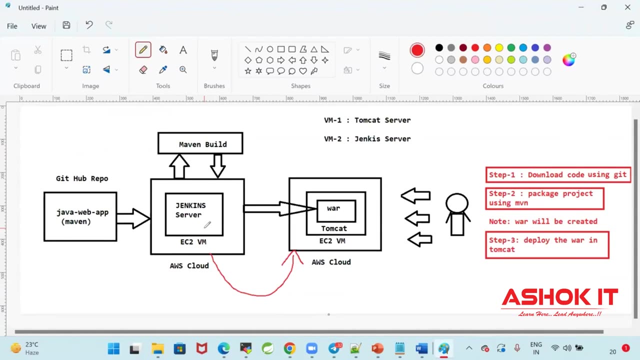 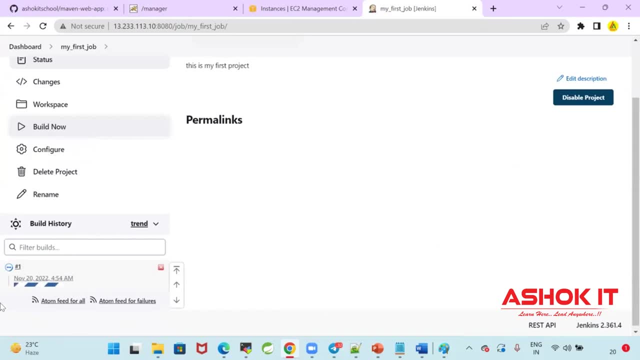 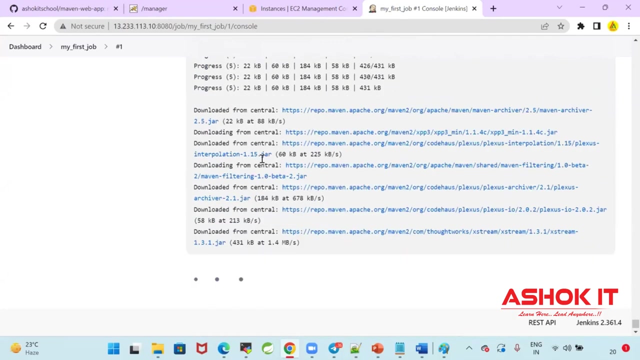 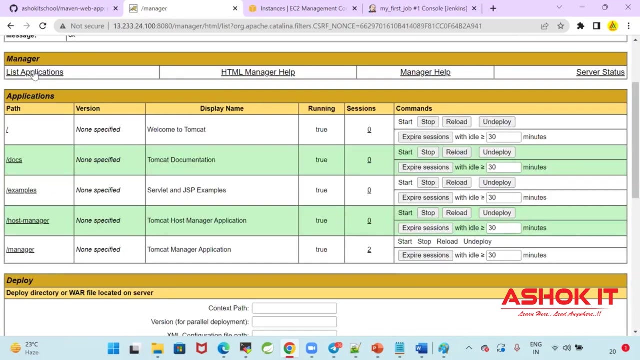 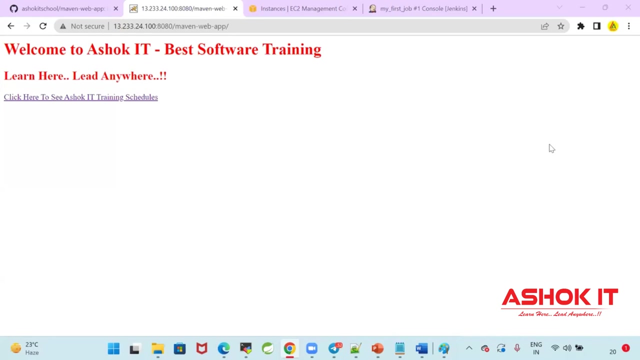 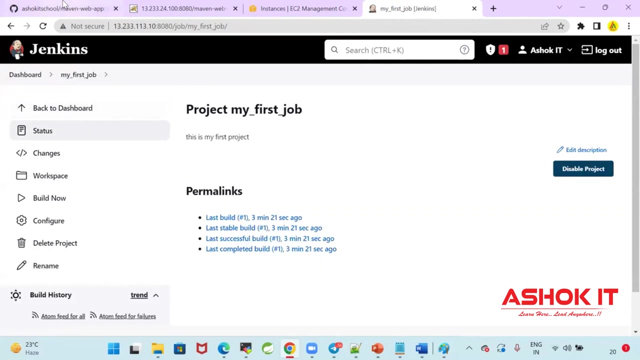 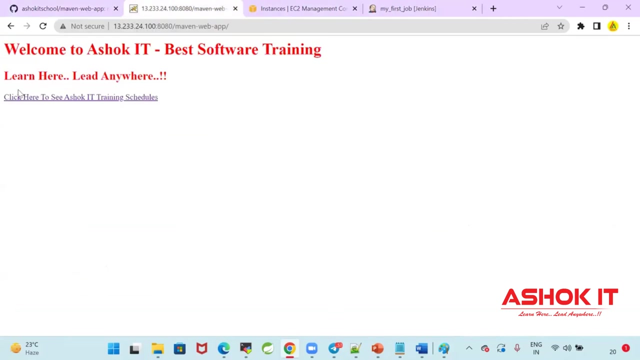 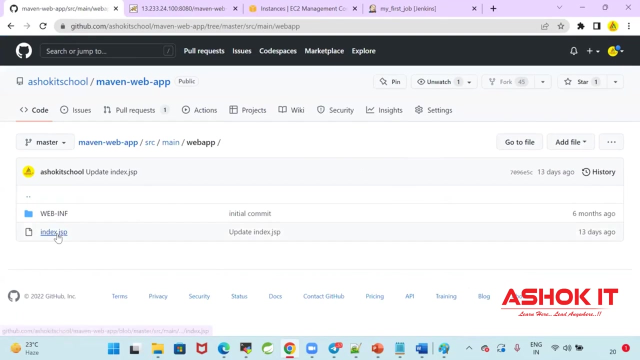 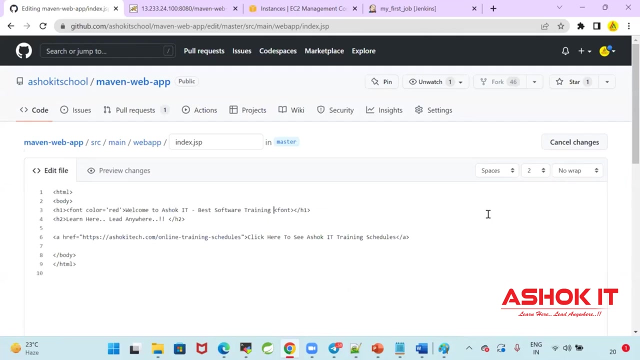 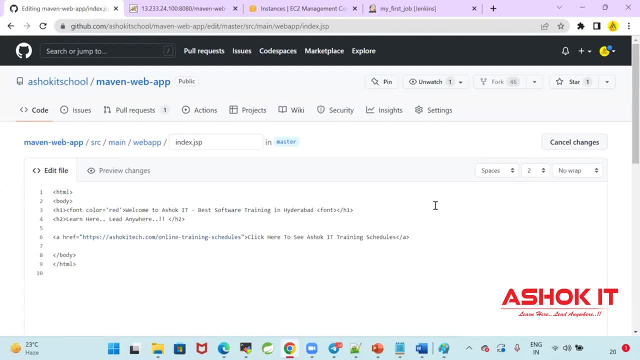 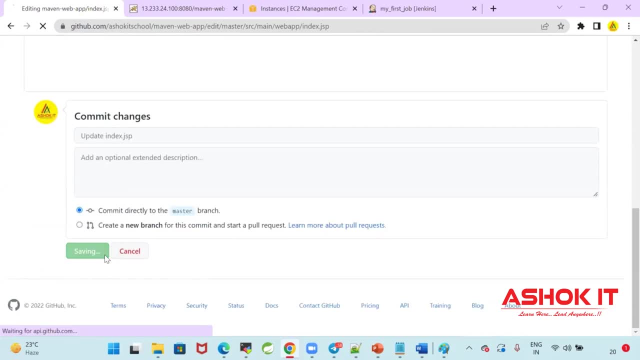 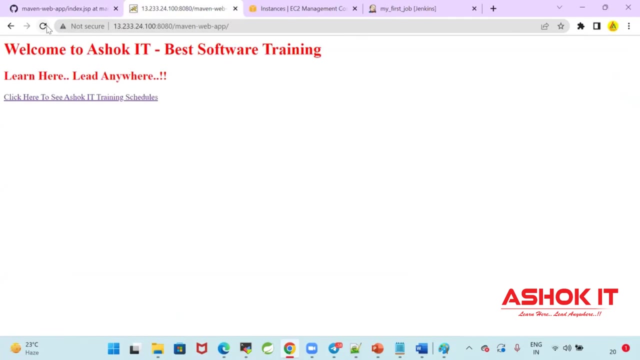 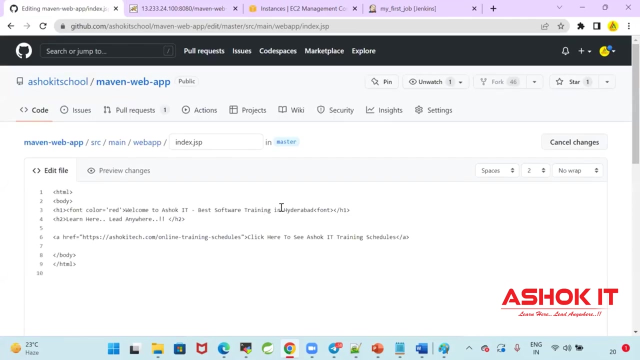 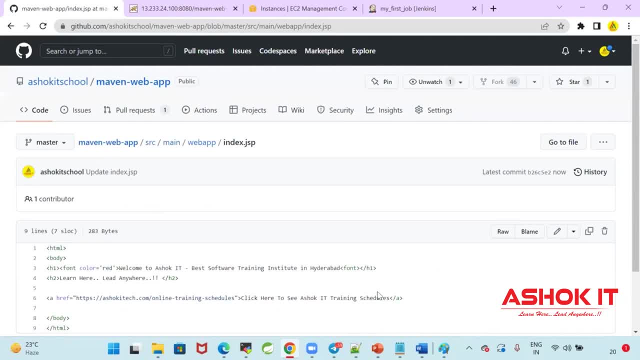 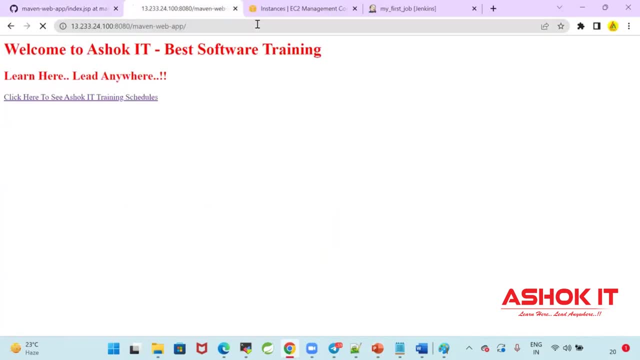 I have done the code changes as a developer. I have done the code changes as a developer. guys, When I do the code changes as a developer, is that code deployed in the server or my code is not deployed in the server? I have done the code changes in the GitHub. 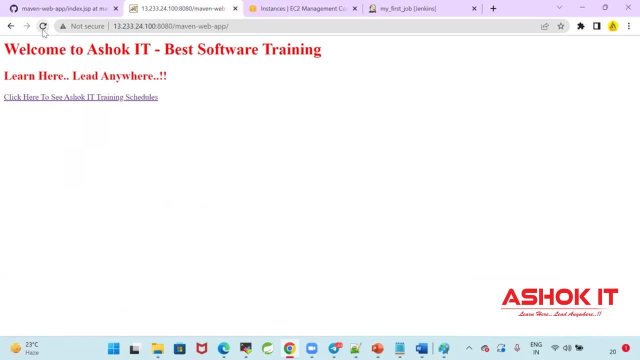 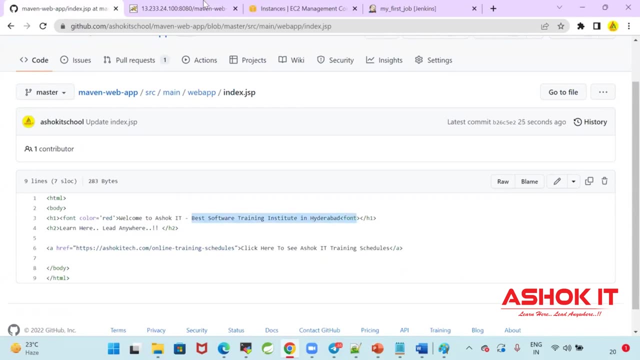 Is the latest code deployed in the server? Latest code is not deployed in the server. No, Actually, content should display best software training institute in Hyderabad. But what is displaying? Just displaying best software training. So my code is not deployed.